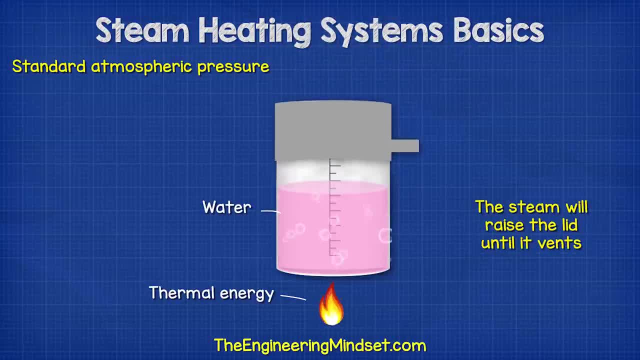 The thermal energy is carried away by the steam. If we capture and contain the steam by placing a loosely fitting lid over the vessel, we would see the lid rise up. If we fix the lid firmly to the vessel, we would see the internal pressure increase. 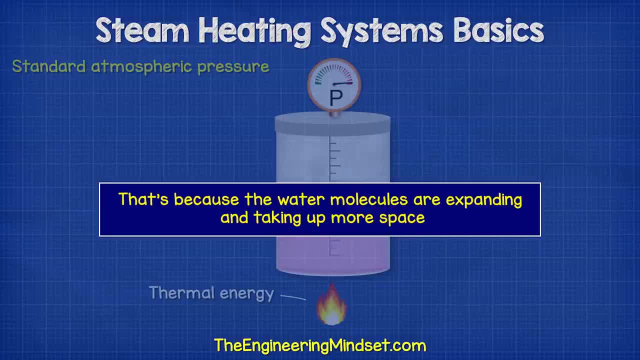 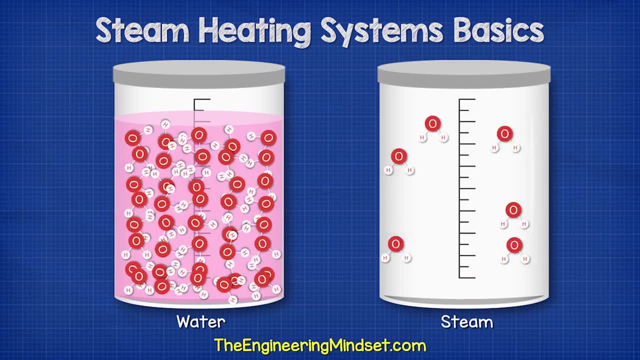 That's because the water molecules are not as hot as the steam. The thermal energy is added to the steam and the water molecules are expanding and taking up more space. In cool water the molecules are tightly packed together, But as more thermal energy is added, the water molecules become excited. 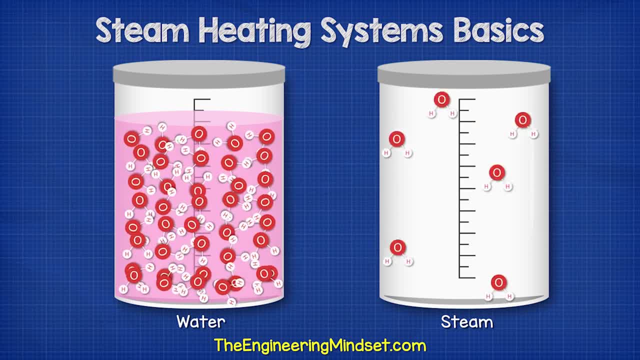 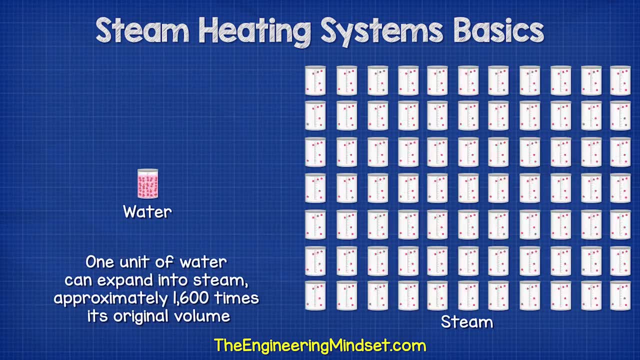 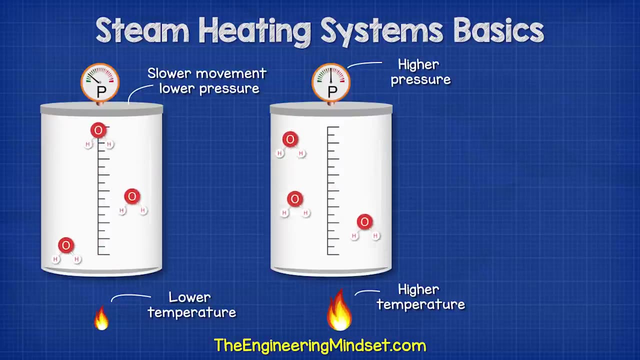 and they vibrate rapidly, which increases their volume. It increases so much that one unit of water can expand into steam approximately 1,600 times its original volume. If the volume of the vessel is fixed and more thermal energy is added, the water molecules are going to become excited and move faster. 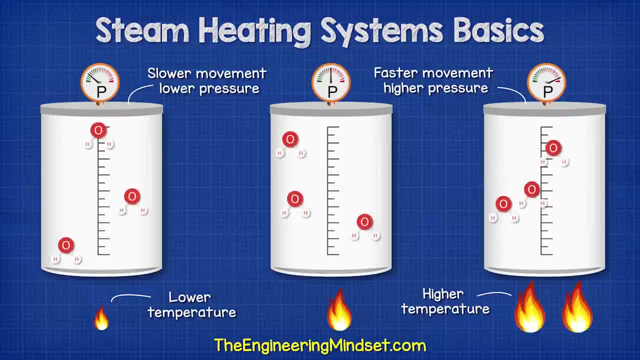 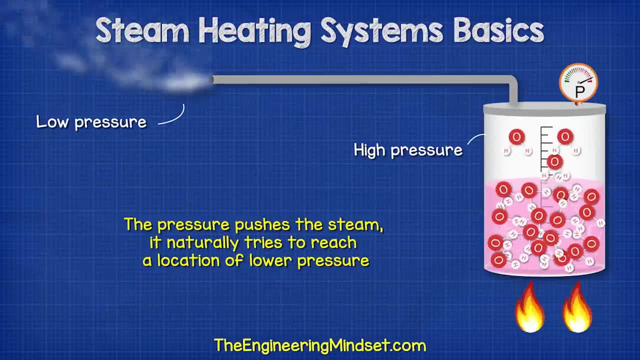 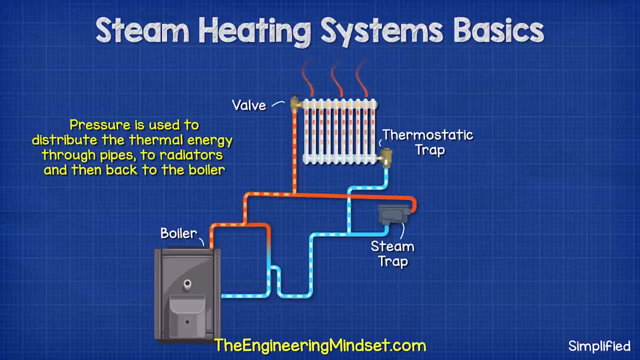 They will collide with the walls of the vessel more frequently and with more force. This increases the pressure inside the vessel. The pressure pushes the steam. It naturally tries to reach a location of lower pressure. We can use that pushing force to distribute the thermal energy through pipes to radiators and then back to the boiler. 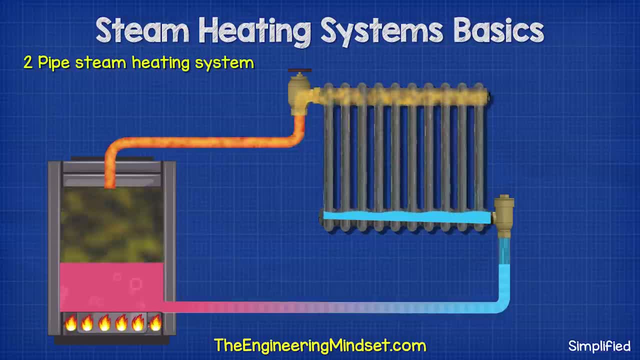 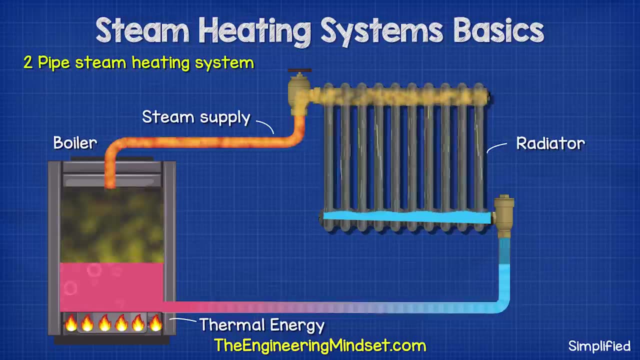 In a typical two-pipe steam heating system, the boiler is adding thermal energy and heating the water, which turns it into steam. The pressure is pushing the steam along the pipe into the radiator. The radiator heats the ambient air of the room, so the thermal energy is transferred from the steam through the radiator wall and into the air of the room. 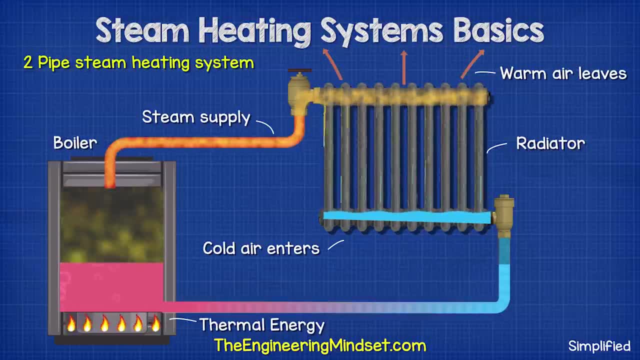 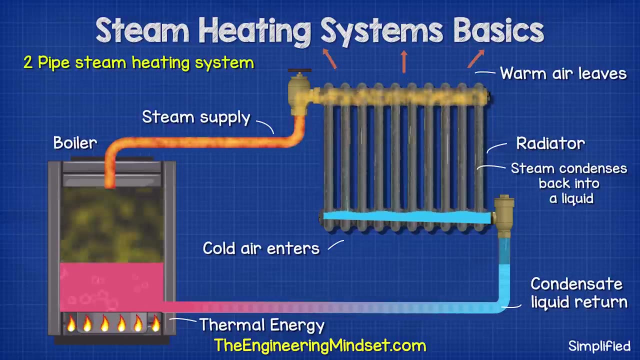 As the air is heated, it rises up and cooler air then rushes in to take its place. This will repeat continuously. The steam is giving away its thermal energy. As it does, so it condenses back into a liquid. The high pressure of the system is going to push this water back to the boiler. 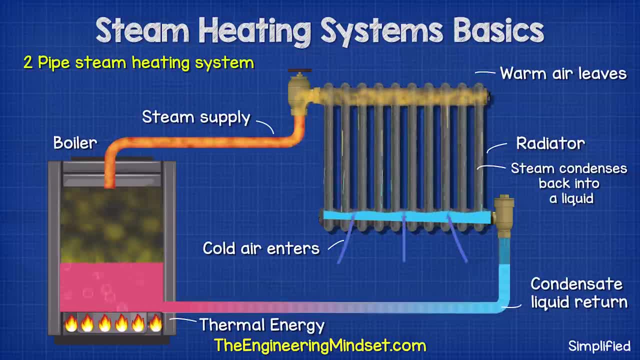 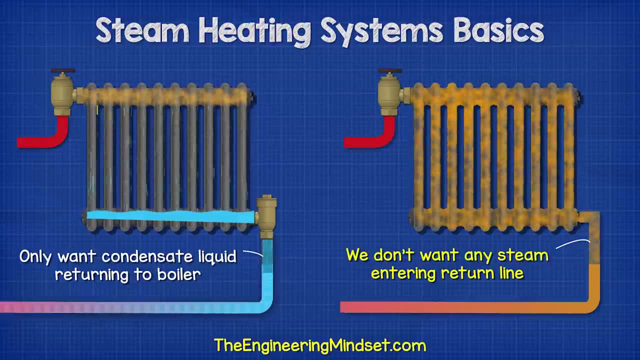 where it will be reheated and repeat the cycle. We only want condensate liquid returning to the boiler. We don't want any steam getting into the return line. This would be a waste of energy as it will warm the condensate liquid. 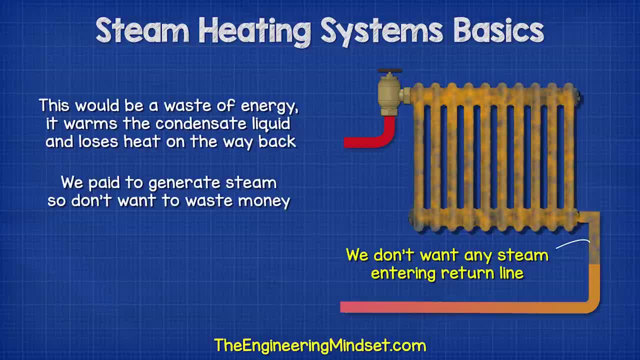 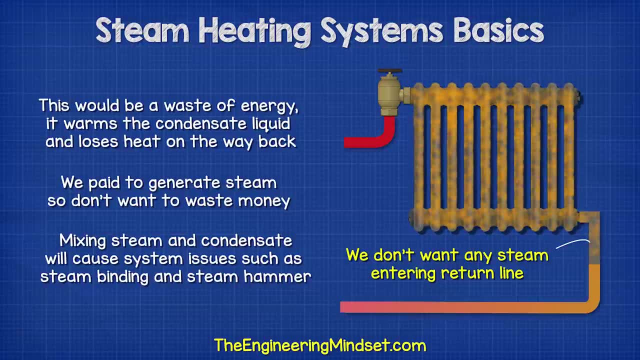 and also lose heat on the way back. We've paid to create the steam, so we don't want to waste it. Mixing the steam and the condensate will cause many problems for the system also, such as steam binding and also steam hammer. 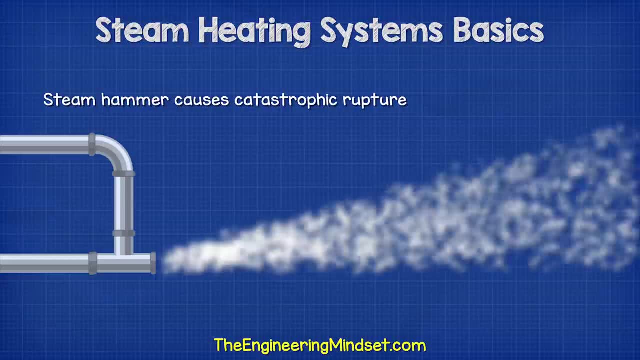 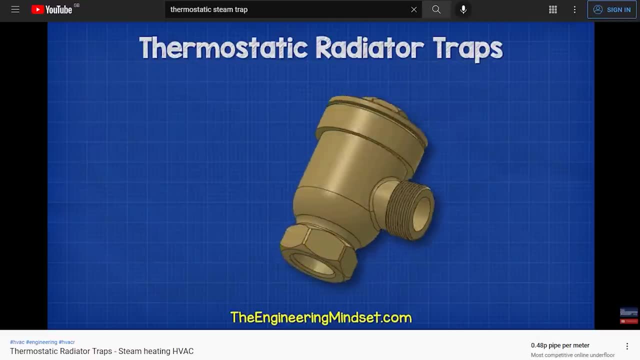 This can be catastrophic for the system, so we must try to avoid this. One way to do that is through a thermostatic radiator trap. By the way, we have covered that in detail in our previous video. Do check that out. Links can be found in the video description. 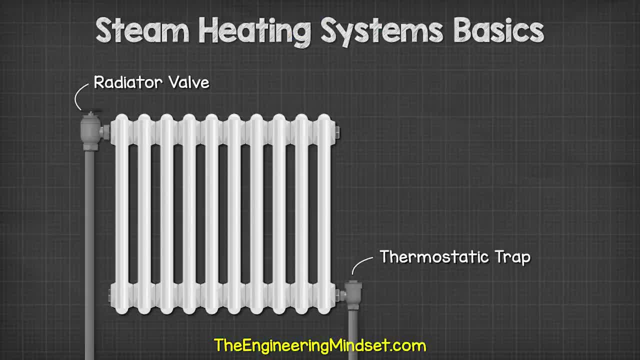 The link is down below. Ok, that's it for this video, but to continue learning about heating systems and engineering, check out one of the videos on screen now and I'll catch you there for the next lesson. Don't forget to follow us on Facebook, Twitter, Instagram, LinkedIn. and, of course, TheEngineeringMindsetcom. 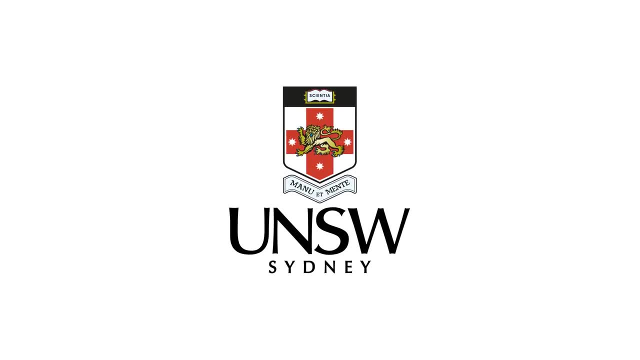 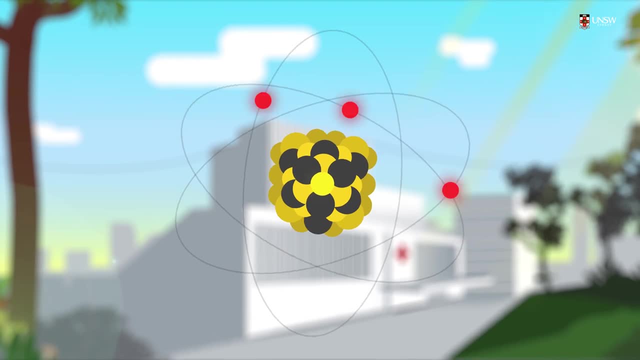 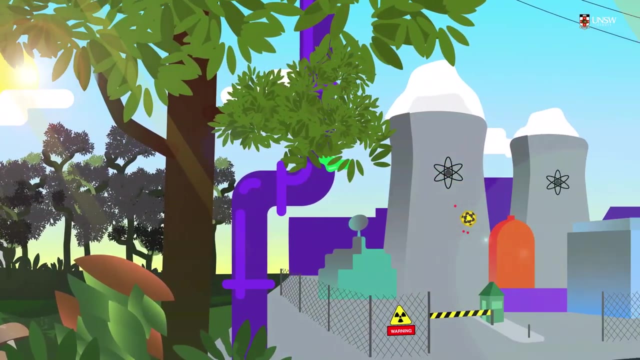 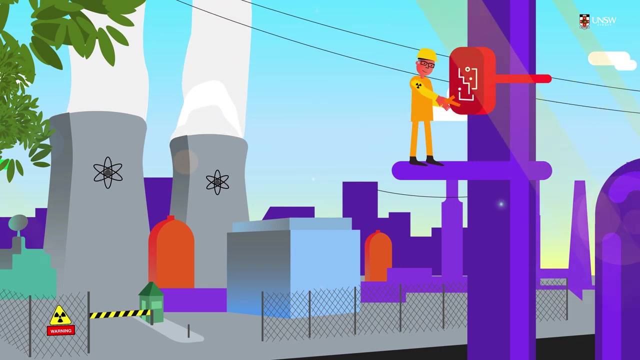 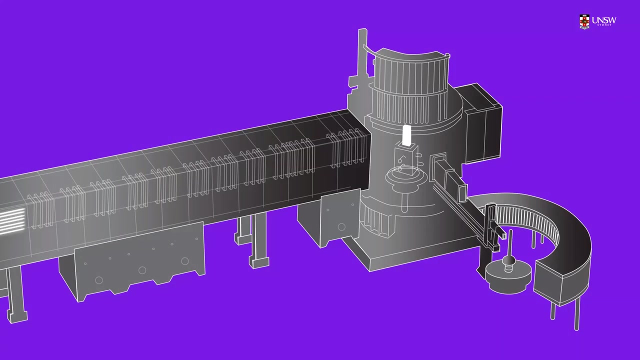 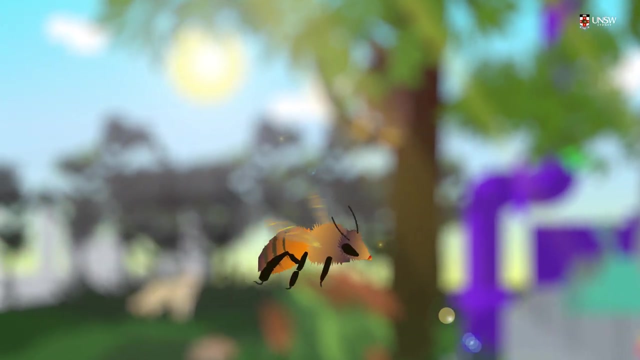 We use radioactive isotopes in medicine. we use them for nuclear energy. we use nuclear radiation for non-destructive testing in engineering and in many fields of scientific research, such as radioisotope labeling and neutron or x-ray diffraction. We are also surrounded by natural radiation every day, from the 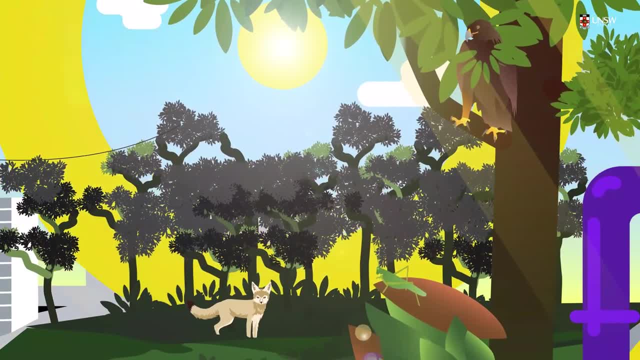 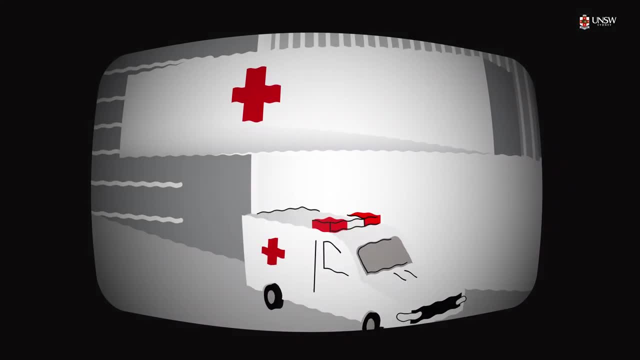 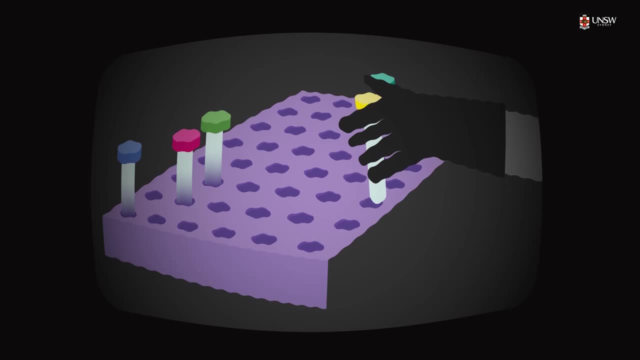 Earth's crust and from the Sun. Unfortunately, small amounts of radiation are harmless, but large amounts of radiation can be very dangerous. Added to this is the possibility that nuclear technology can be diverted to non peaceful purposes. What do we do to ensure that our safety and our security? 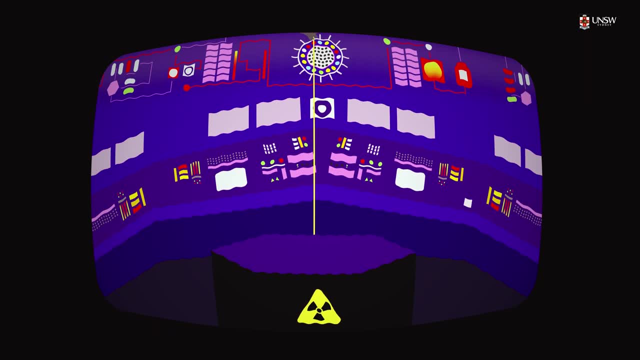 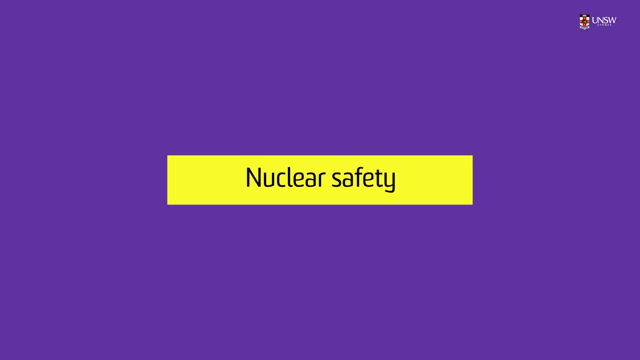 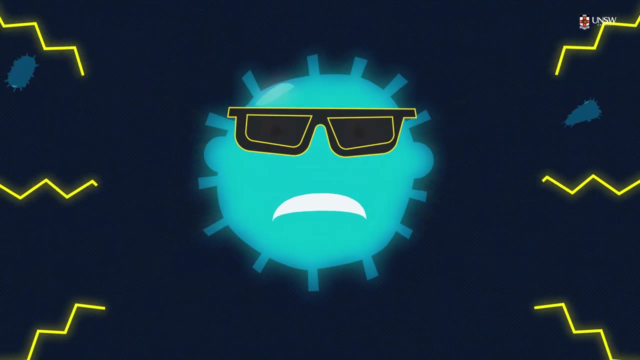 are not compromised by the promise of nuclear technology, and how do we guarantee that nuclear materials are used only for peaceful purposes? One nuclear safety Harm from radioactive materials can occur as a result of direct exposure to ionizing radiation, and it can occur from ingestion of